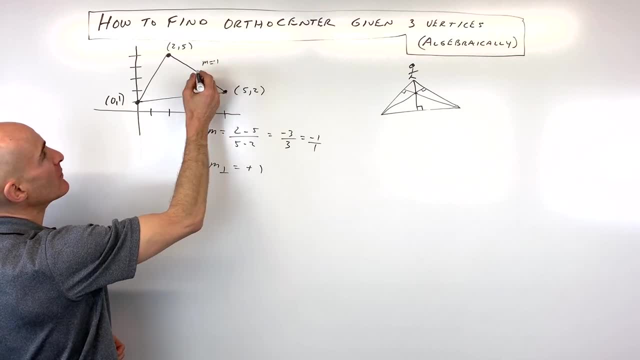 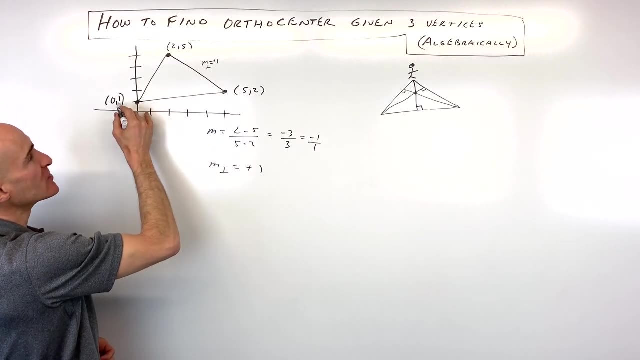 We'll just write slope of negative one, but this is going to be a positive one which is going to be the perpendicular slope. We know that the line is going to go through the point zero one. So if we look at this line here, you can see that the y intercept is going to be one and it's going to 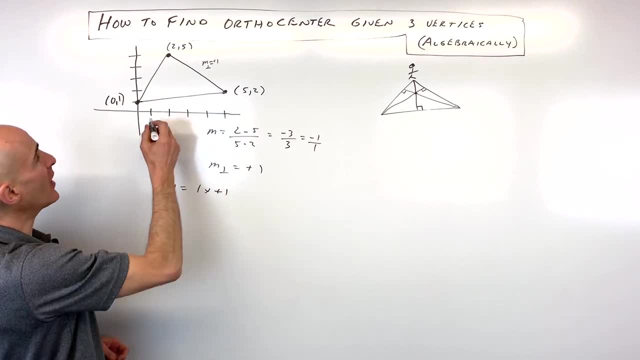 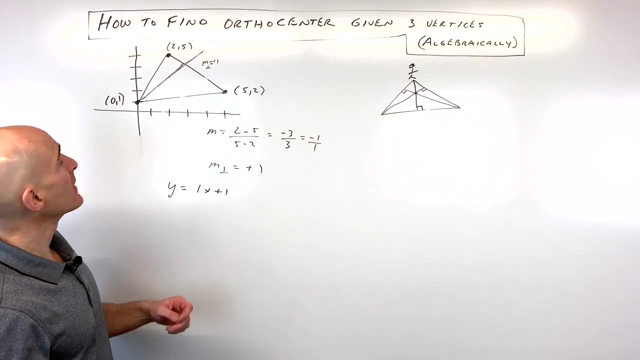 have a slope of one. So our equation is: y equals one, x plus one. So that's going to look something like: let's see: up one over one, up one over one, up one over one, etc. So it's going to look something like that. My diagram is not perfect, but that's the basic idea there. Now let's go ahead and find. 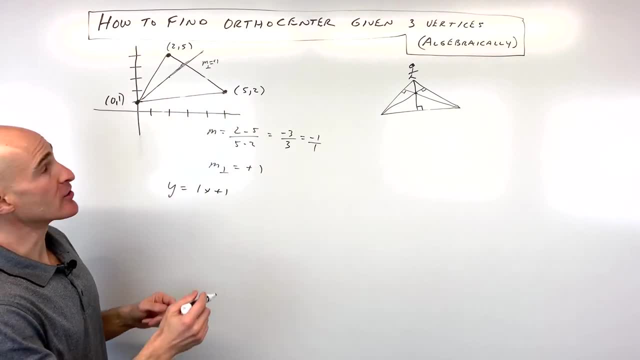 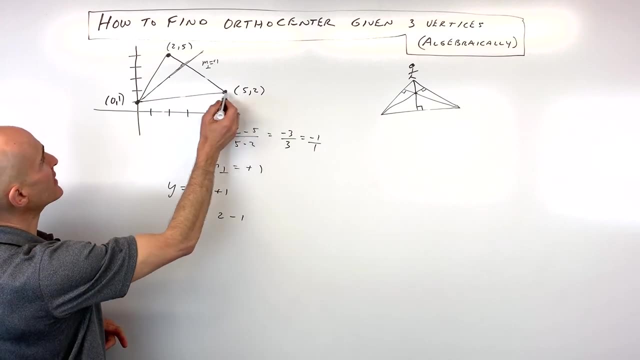 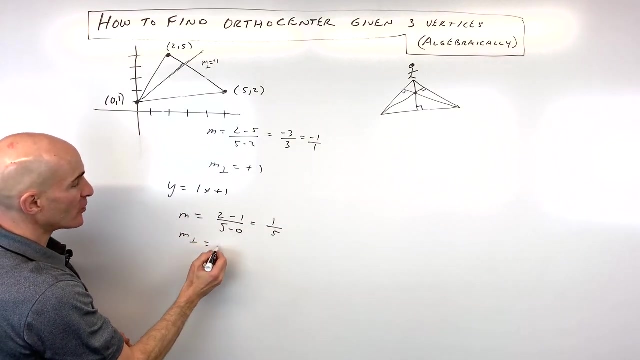 the altitude from this point to this opposite side here. So we want to find the slope of this line, so that's going to be one which is two minus one, and x, two minus x, one, which is going to give us five minus zero, So that gives us one fifth. Now the perpendicular slope is going to be negative five. 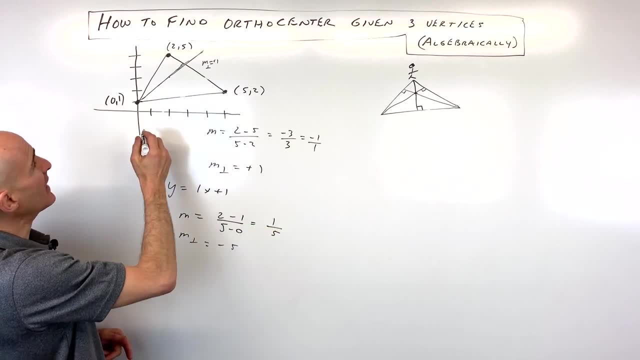 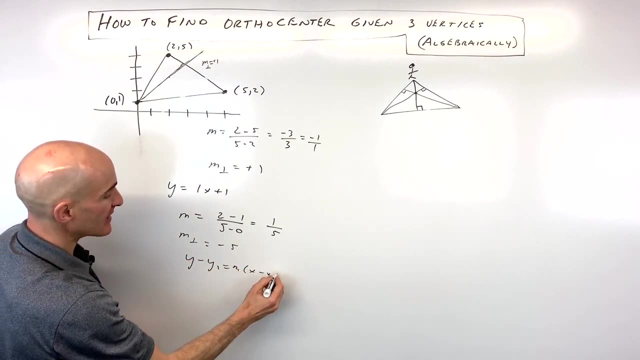 because I'm flipping that over and making it the opposite sign, And here you can see it's going through the point two five. So what I'm going to do is I'm going to use the point slope form: y minus y one equals m times x minus x one. We know that the slope is negative five. It goes through the. 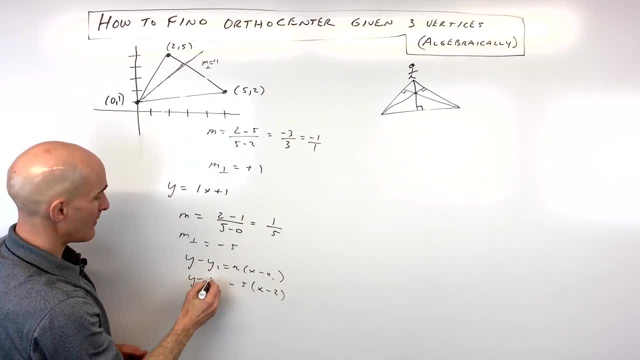 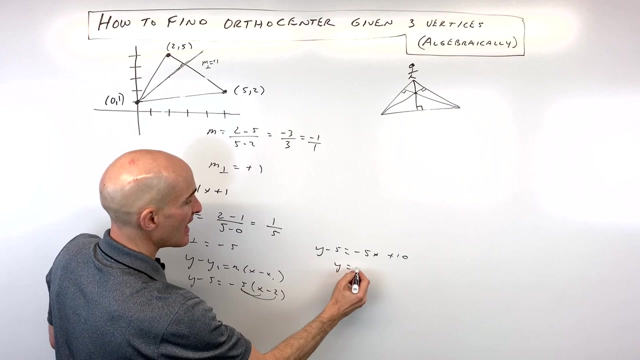 point two, five. So x minus two, y minus five. And we can simplify this a little bit by distributing the negative five. That's going to give us y minus five equals negative five, x plus 10 plus 10.. And if I add five to both sides, 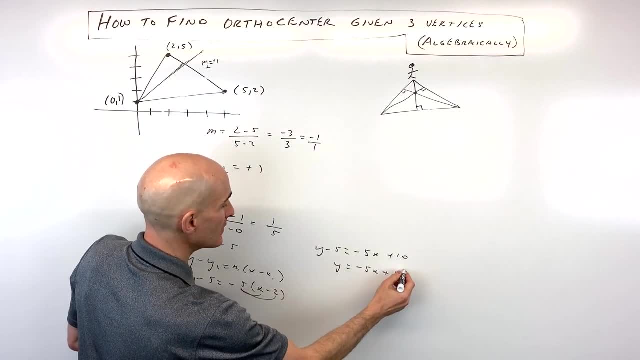 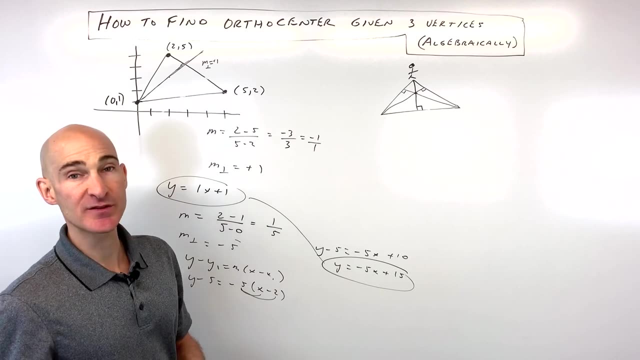 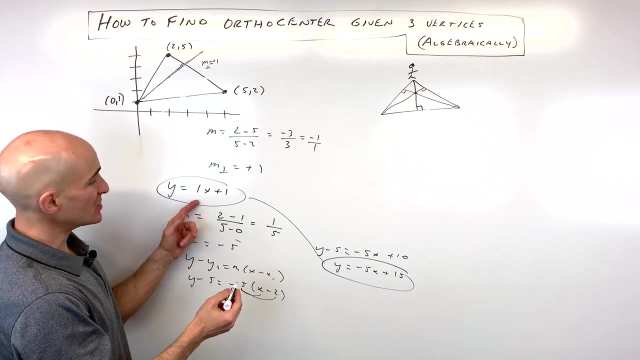 we get negative five x plus 15.. Okay, so now you can see we've got two equations here: y equals one x plus one, and y equals negative five x plus 15.. We just have to find the point of intersection of y and x. So what we need to do here is we need to do a substitution: y equals one x plus one. I'm 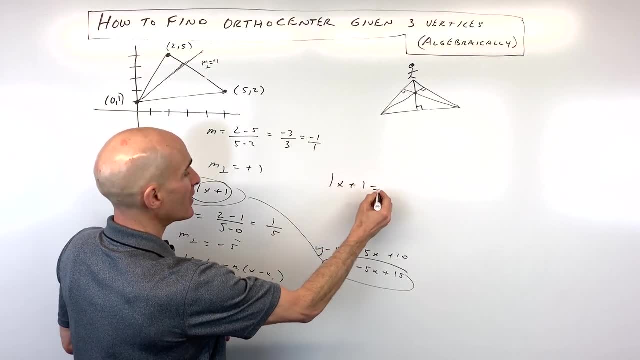 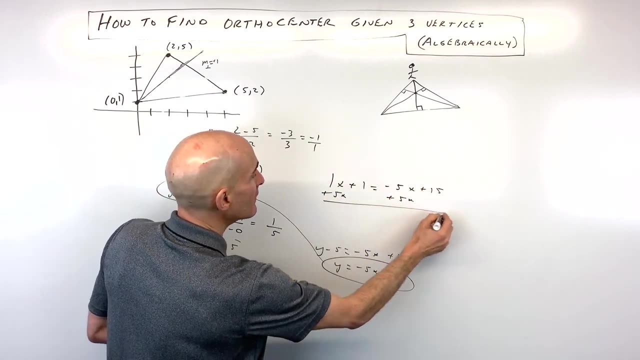 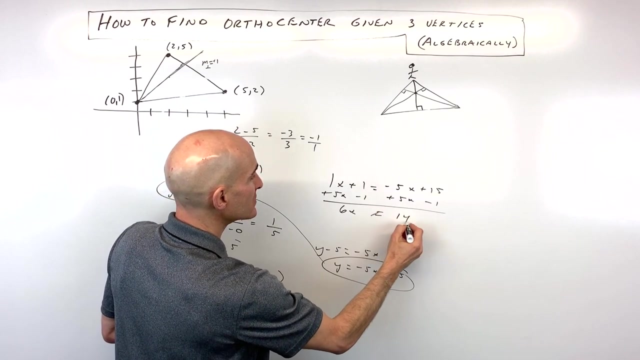 going to put that in place of y here. So we have: one x plus one equals negative five x plus 15.. If I add five x to both sides, that gives us six x, And if I subtract one from both sides, that gives us 14.. And if I divide by six, x equals 14, six, which equals seven thirds. if you reduce.